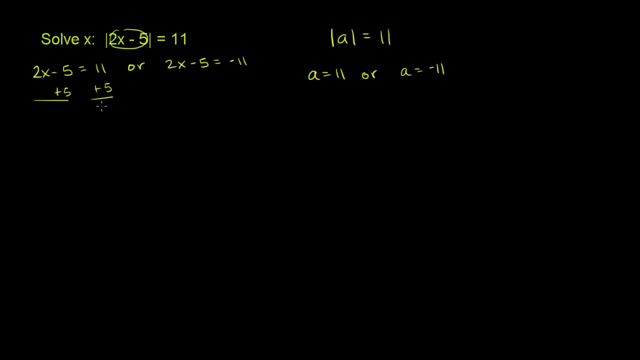 So both sides of this equation we get: 11 plus 5 is 16.. 2x minus 5 plus 5 is just 2x. 2x is equal to 16.. Divide both sides by 2.. We get x is equal to 8.. 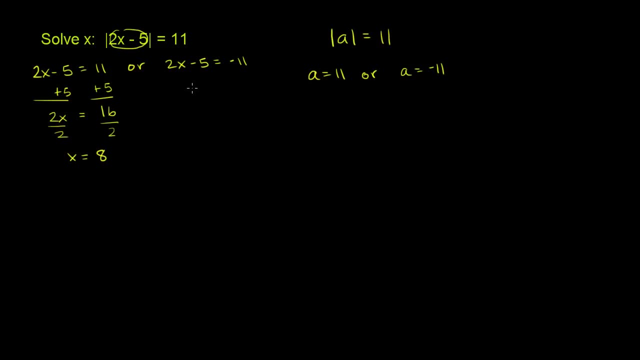 Now let's do this situation: 2x minus 5 is equal to negative 11.. Let's add 5 to both sides of this equation, The left-hand side, we just get a 2x. The 5's cancel out. 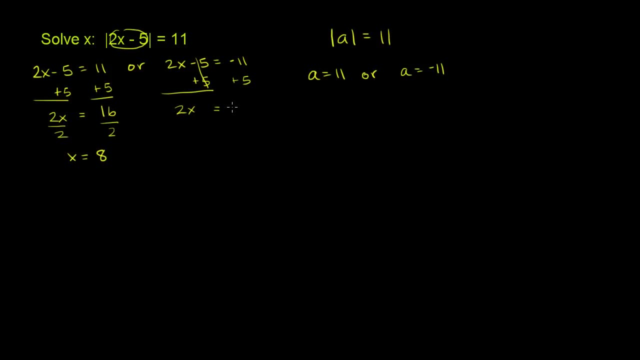 2x is equal to negative 5. Negative 5 plus 11. That's negative 6.. Now we can divide both sides by 2. Divide both sides by 2. And we get x is equal to negative 3.. 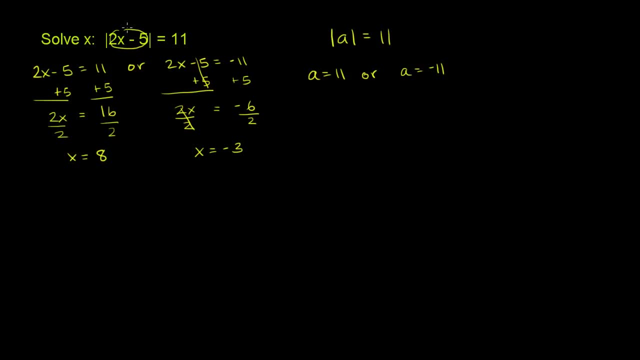 So we've gotten two solutions, depending on whether this thing in here is either equal to 11 or negative 11.. We got x could be equal to 8, in which case 2x minus 5 would be 11.. Or we have x is equal to negative 3,. 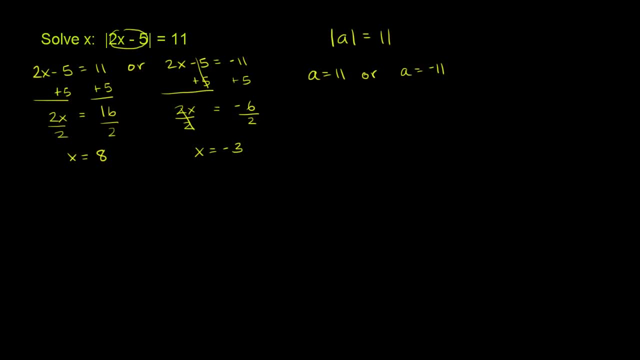 in which case 2x minus 5 is equal to negative 11.. Let's verify it. So if x is equal to negative 3, then 2x minus 5 is equal to negative 11.. So if x is equal to negative 3, then 2x minus 5 is equal to negative 11.. 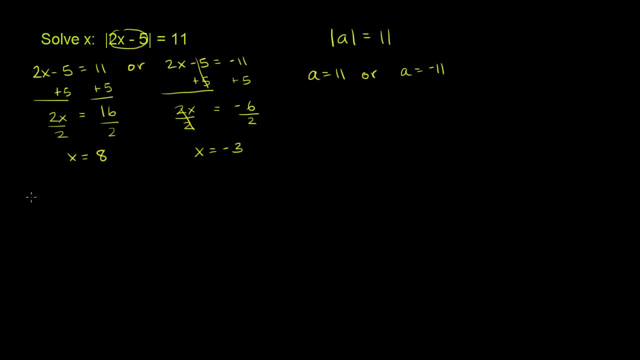 Let's show that it satisfies this equation. So we'd get 2 times 8 minus 5.. The absolute value of 2 times 8 minus 5 should be equal to 11.. 2 times 8 is 16, minus 5 is 11.. 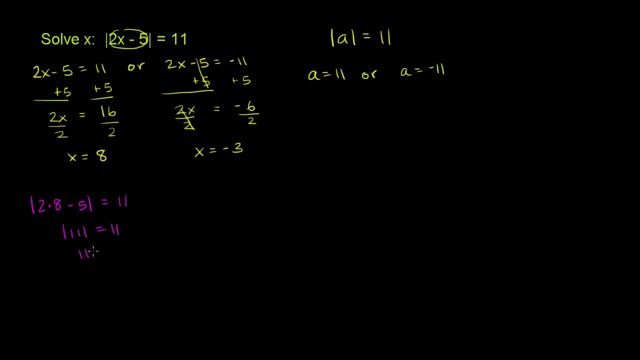 So we have: the absolute value of 11 should be equal to 11. And we know that's true. The absolute value of 11 is 11.. So it all works out. Now let's try it with: x is equal to negative 3.. 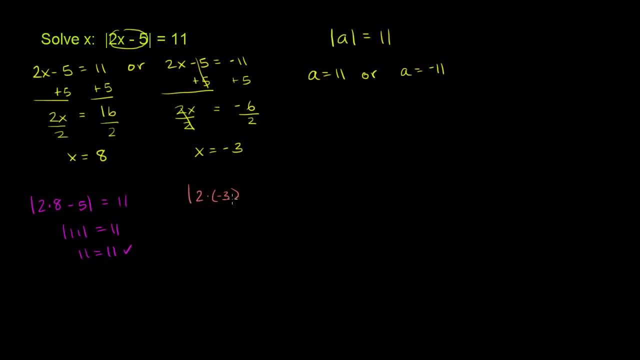 We get the absolute value of 2 times negative 3 minus 5 should be equal to 11. to 11.. So what's 2 times negative 3?? 2 times negative 3 is negative 6 minus 5.. The absolute value of that should be equal to 11.. 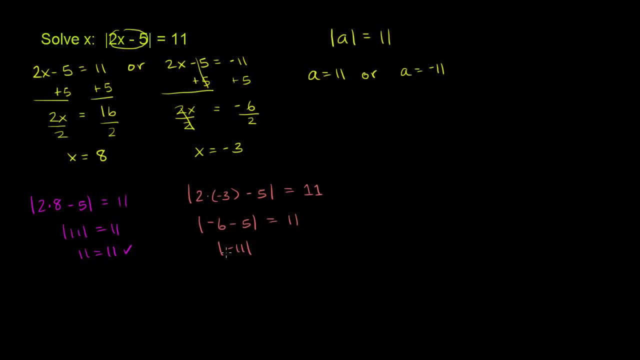 Well, negative 6 minus 5 is negative 11.. So the absolute value of negative 11 should be equal to 11. And it is The absolute value of negative 11 is 11. So we get 11 is equal to 11. So they both work.